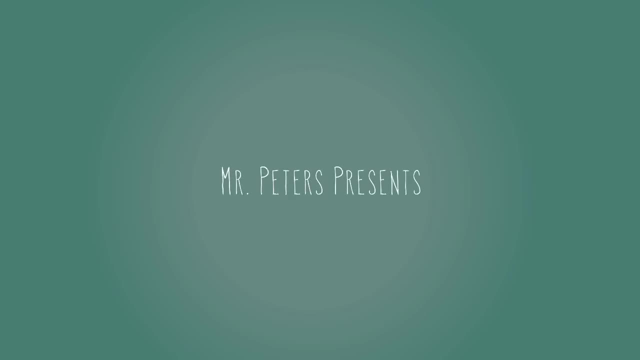 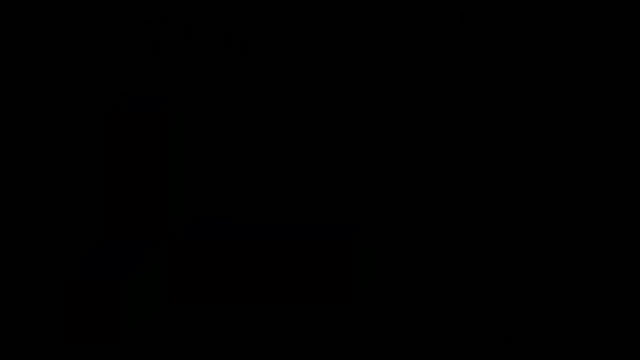 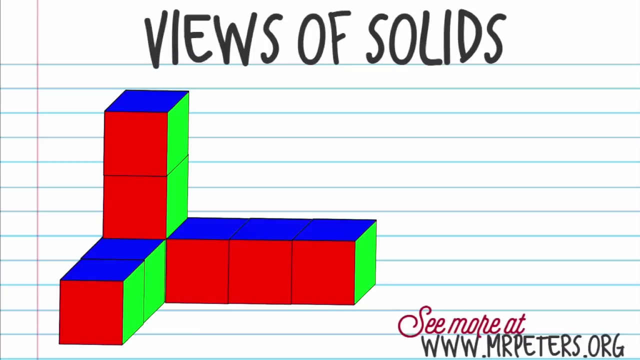 Today we're going to talk about the views of solids. When we think of views of solids, we're looking at three dimensional figures. So we have our cubes here stacked. We have eight cubes stacked on top of each other. We have one, two and there's one back here. 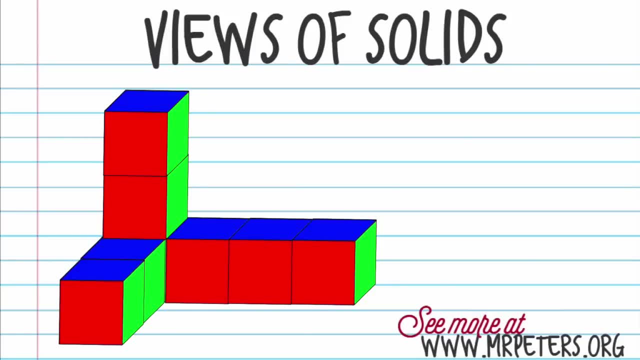 that you can't see. So that's three, four, five, six, seven, eight. And when we're dealing with views of solids, we're going to talk about three views. Views we're going to talk about are side view, top view and front view. The side view would be the green, the top view 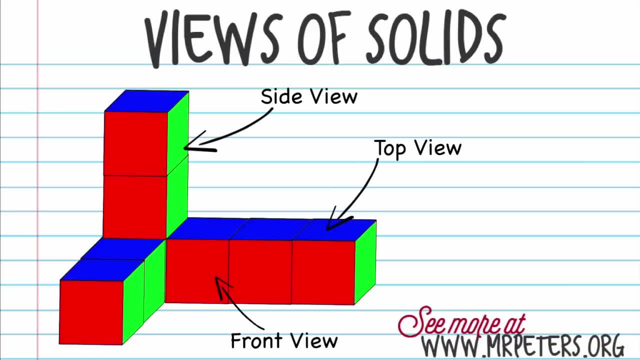 would be the blue and the red would be the front view. So what that means is, if you're standing up here, you're only going to see the red, But if you're standing over in this area, you're going to see the green, And if you're up here somewhere you're probably only 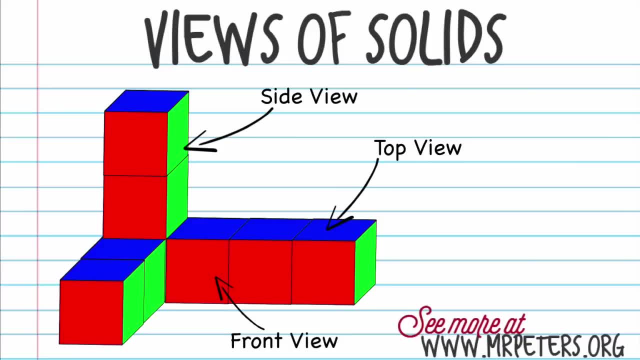 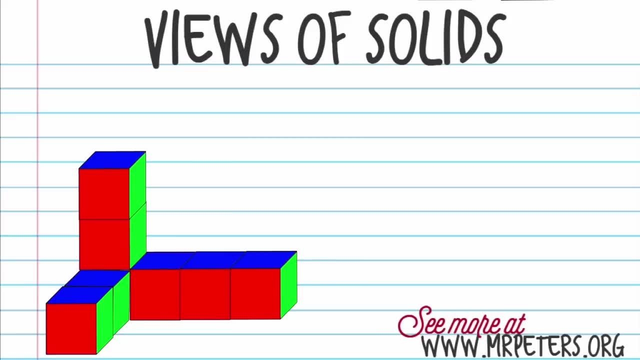 going to see the blue, So how can we draw that out? When we're drawing this out, we're using three different, three separate drawings to look at this. Okay, so now we're first going to start with our front view. So just imagine that we're standing in front, but we can only 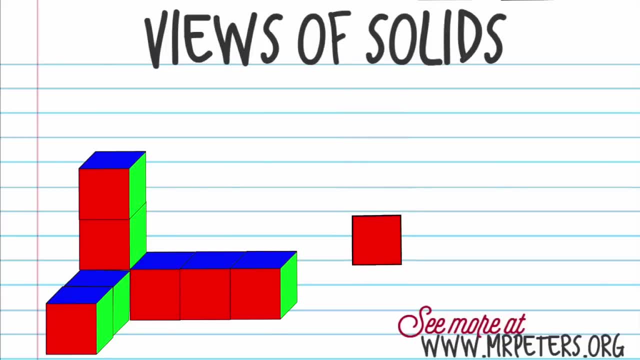 see the red First. we're going to put our one out here to represent this one, And if we're looking at it just at the red, we see that we would think that we would see three red stacked on top of each other. So that's what I'm going to do: One, two, three. Okay, So we have our. 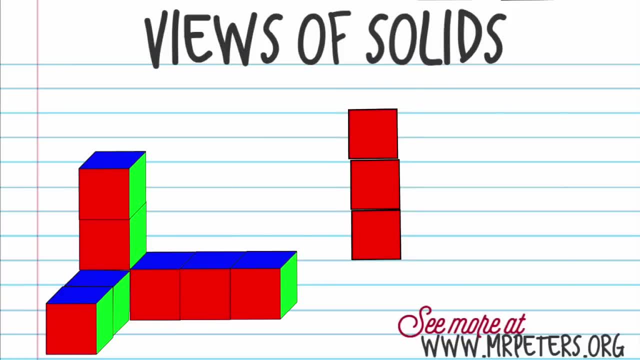 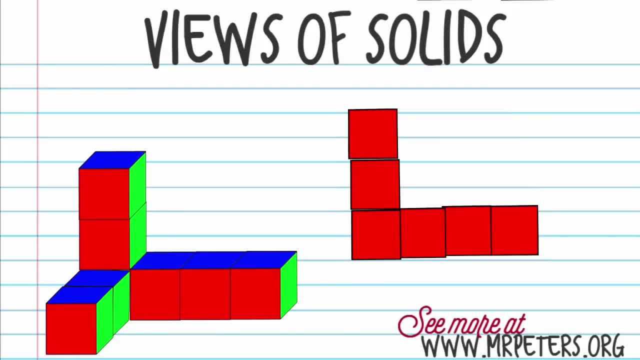 it. we see one, two, three, four over, One, two, three, four over, And one, two, three up. So again, that is our front view. Now let's look at our side view. Remember, our side view is in green, So let's look at the green. That's a map.